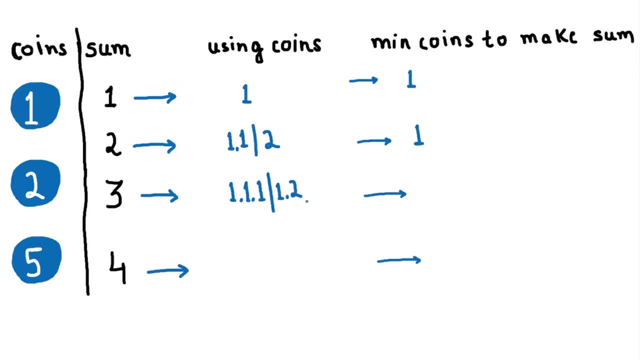 Or we can use coin 1 and 2.. So the minimum coins to make that sum will be 2.. Now we want to make a sum of 4, so we can use coin of denomination 1- 4 times. Or we have another option, like we can use coin of denomination 1- 2 times and coin of denomination 2- 1 times. 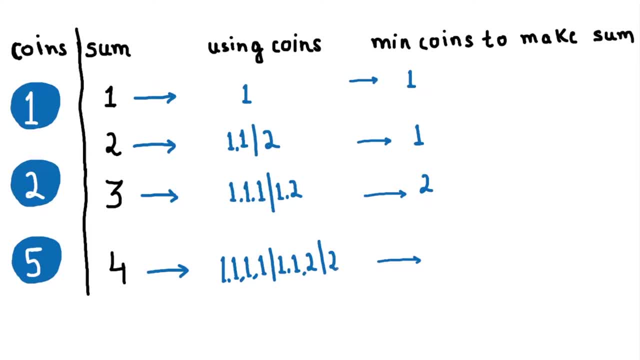 Also, we want to make a sum of 5, so we can use a fraction of 5 times, Or we can use coin of denomination two, 2 times, So the minimum coins to make that sum will be 2.. And we can go on to find minimum coins for any sum. 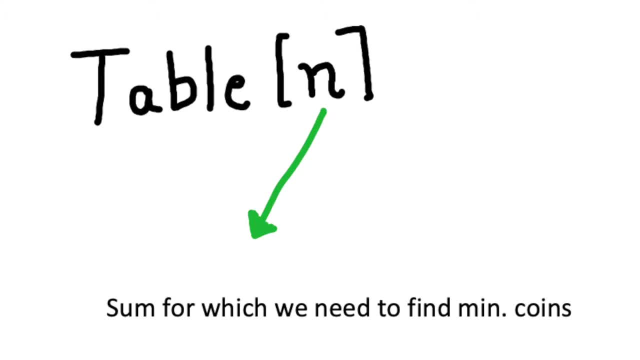 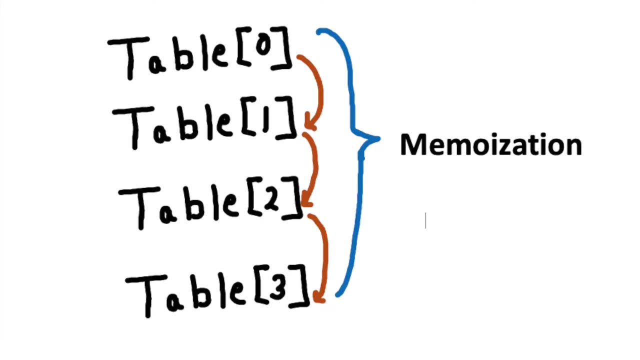 So we will use memorization technique to get the number of coins for any sum. We will take an array and we'll call it table sum. we want to calculate number of coins for and will initialize with max value of integer and we will iterate over sum, starting from 1 to calculate the number of coins, that is. 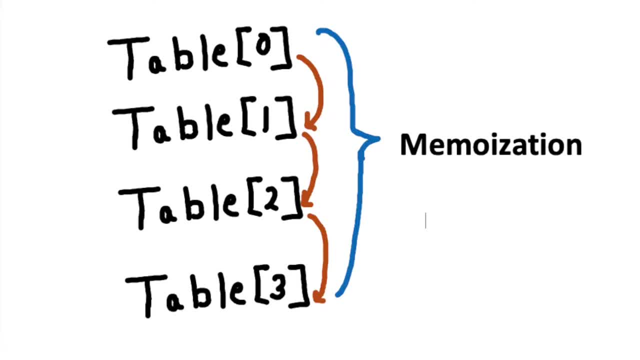 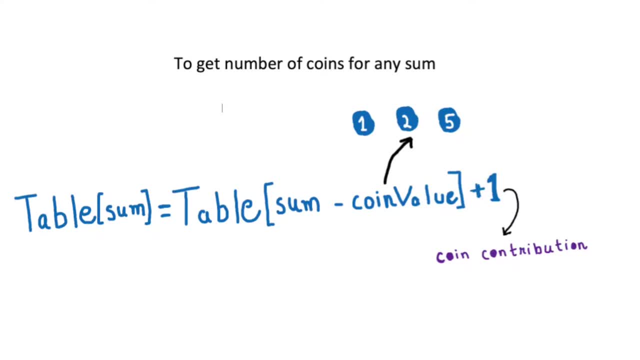 we will calculate number of coins used for sum 1. then we will use its result to calculate for the sum 2.. now the important part, that is, for every sum starting from 1 to end, total coins will be table sum minus of coin value plus of 1, that is total coins used when we subtract current coin. 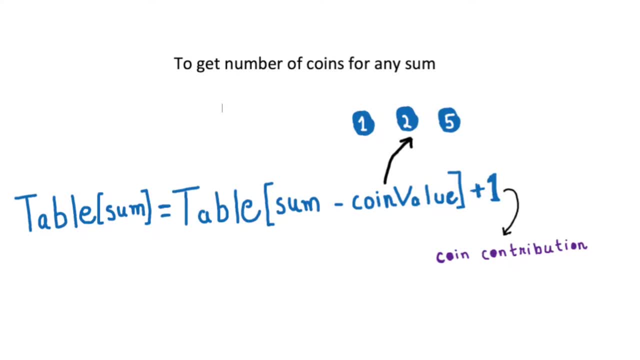 value which can be of denomination 1, 2 or 5 from the sum plus of 1. here we are adding 1 because it is a contribution of that coin which we use to subtract from the sum. let me try to explain this once more with some simple example. let's say we want to calculate total coins used for sum 5. 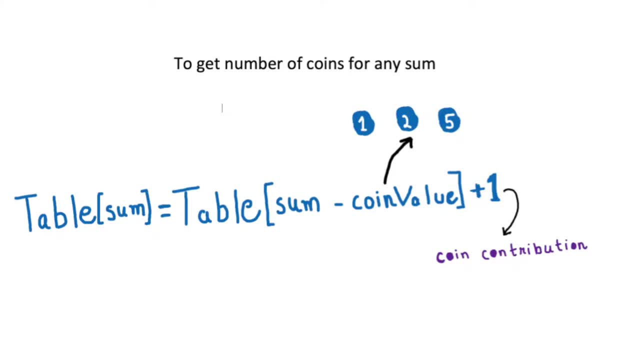 if we have only coin with denomination 1. so it will be table of 5 which will be equal to table of 5 minus of 1 plus of 1, table of 4 plus of 1. so whatever we have in table of 4 plus 1, 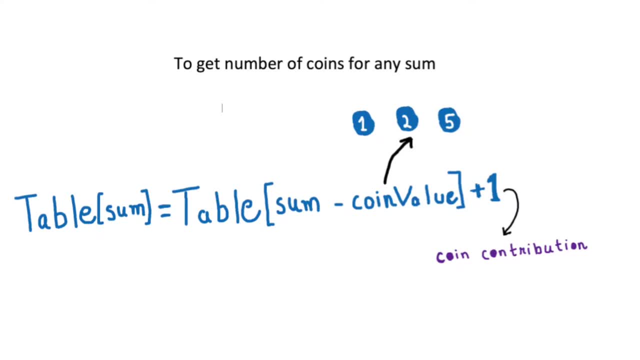 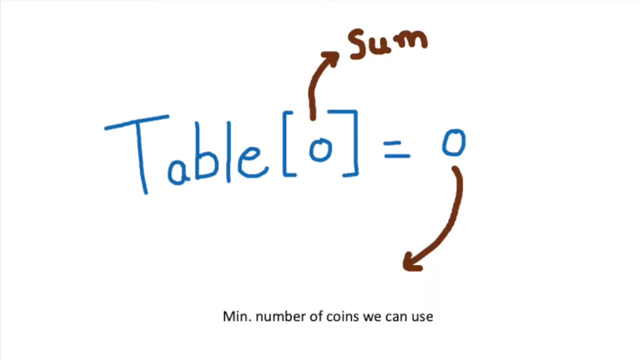 will be our answer for table of 5. and one more thing: as we have multiple coins of different denomination with unlimited supply, we will calculate number of coins for using every combination and get the minimum out of it. for table 0, value is 0, that is, total coins used. 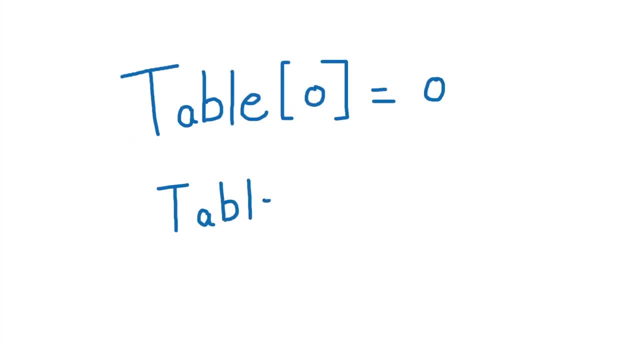 for sum 0 is 0.. for table of 1 it will be table of 1 minus of 1 plus of 1, that is table sum minus of coin value, plus of 1.. here we are using only coin of denomination 1 as using coin of. 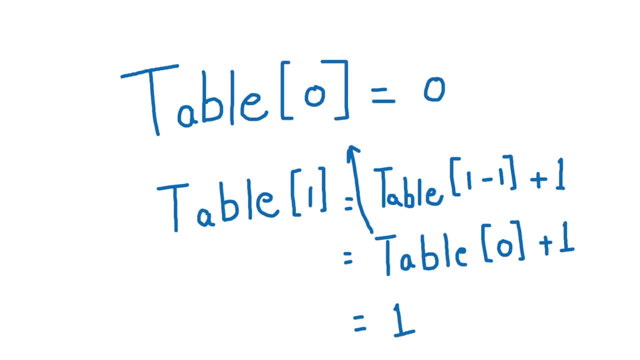 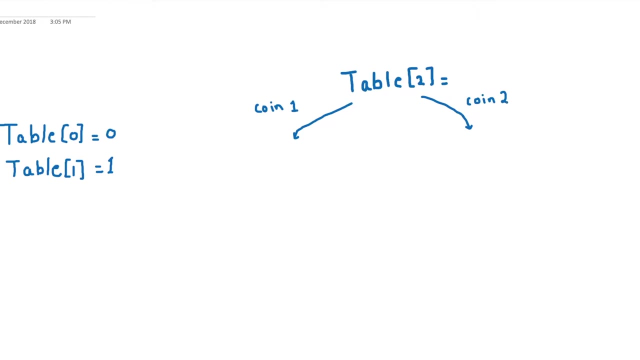 denomination 2 make no sense as coin value of it is greater than the sum itself. for table 2, we have two options. what i mean to say is that we can use coin 1 or coin 2 to make this sum, and we will choose whichever is the minimum one. we can either use coin of 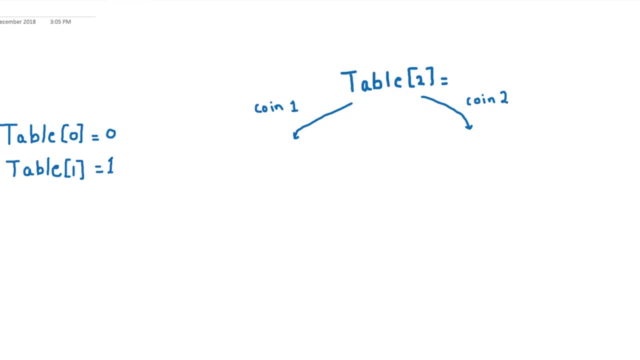 denomination 1 or coin of denomination 2. for both we will use the result that we calculated for table 1, which is the minimum coins we can use to make the sum of 1.. so using coin value, 1 statement will be: table of 2 minus of 1 plus of 1, which makes table of 1 plus of 1. 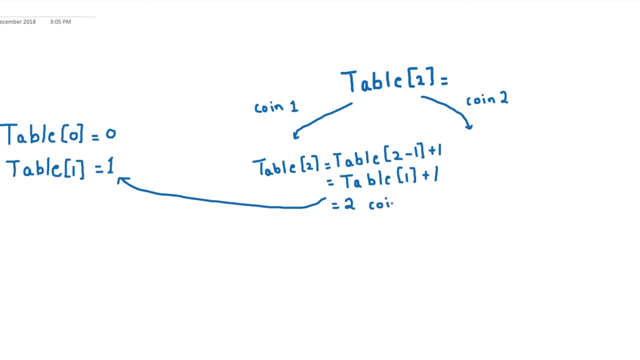 so whatever we have in table of 1, that is 1 and plus of 1 will be a result that is, two coins of denomination 1 to make sum of 2. you can see that plus and minus coordになりました to make table of 2. 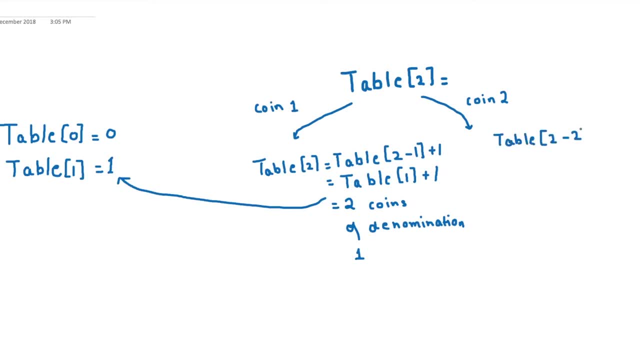 if we use coin value, two statement will be table of 2 plus of 2 or, to usual expressions, the final element of zero and plus of 1, which make 2 plus of two. so whatever we have in table of 0, that is, 0 and plus of 1 will be a result. 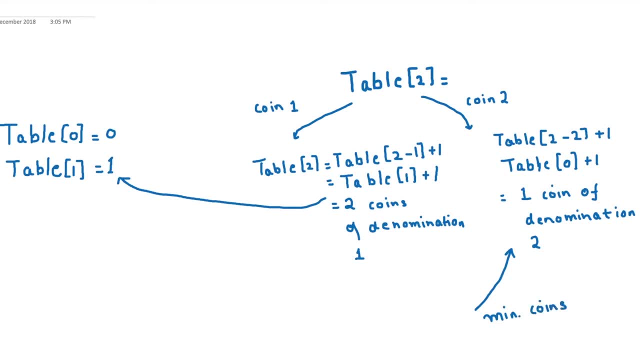 that is one coin of denomination, two to make sum of 2, coins to make sum 2.. Now let's have a look on the pseudo code. So we will loop through the sum from 1 to n and again we will have a inner loop which will loop through the coins.